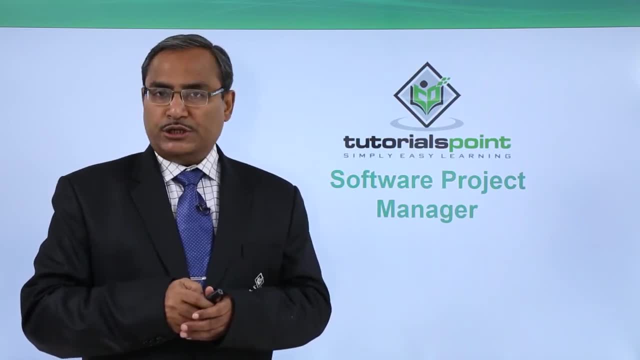 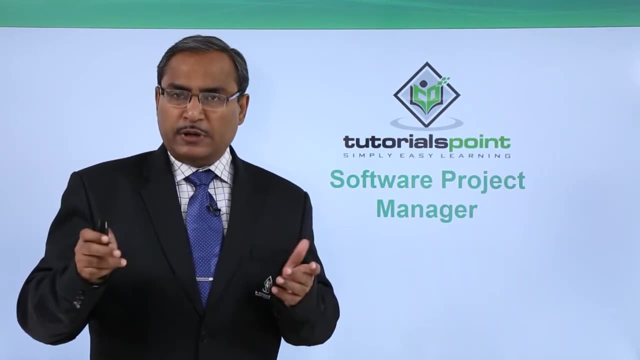 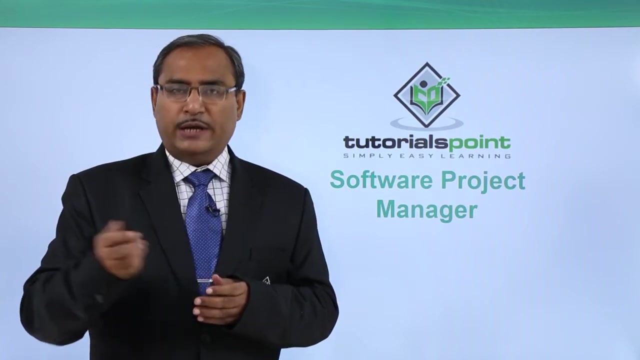 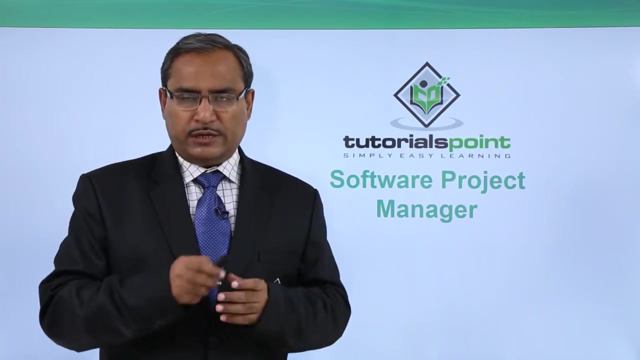 his or her study And this particular software manager. this software project manager will be also establishing a communication between multiple resources and users regarding multiple different issues. There is a budget, cost, the resources, the quality and the user's feedback. So let us discuss the roles and responsibilities of software project manager. 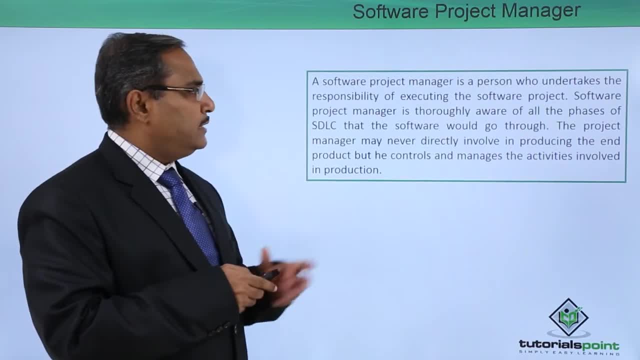 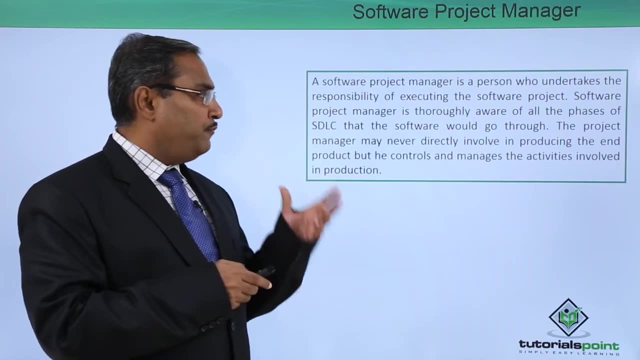 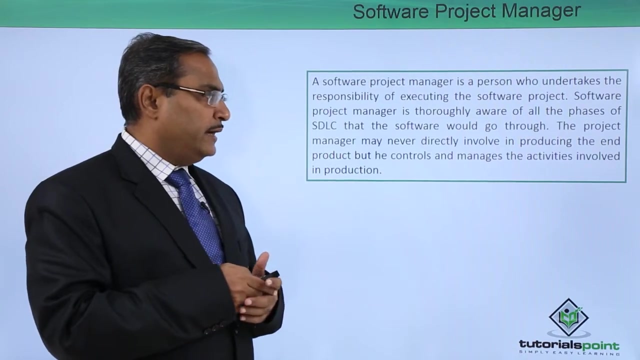 So a software project manager is a person who undertakes the responsibility of executing the software project. The software project manager is thoroughly aware of all phases of SDLC that the software would go through And the project manager may never directly involve in producing the end. 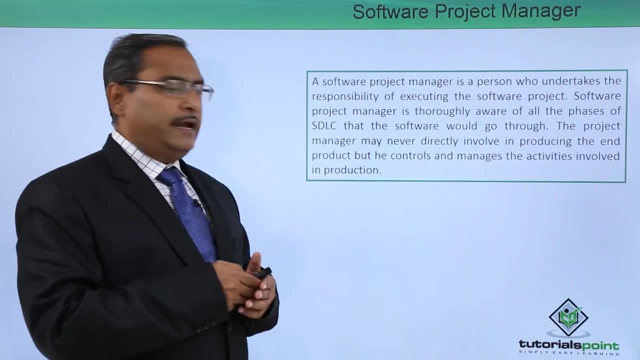 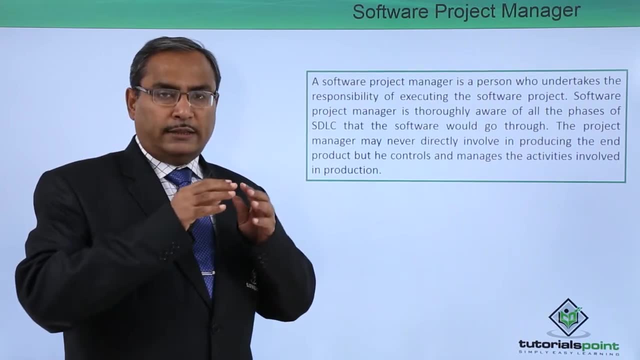 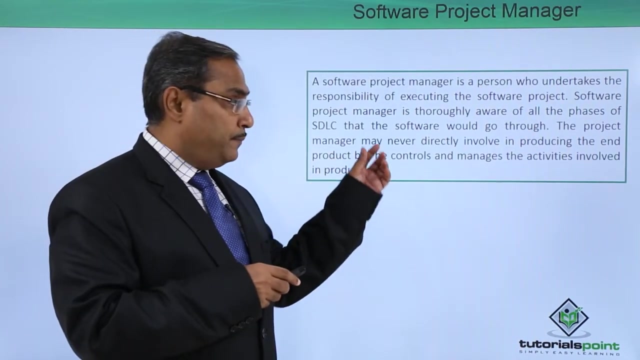 product but he controls and manages activities involving in the production. So this software project manager will do the managing, controlling and this supervising all the activities for this development process. So he might not be involving in the producing the end product but might be. 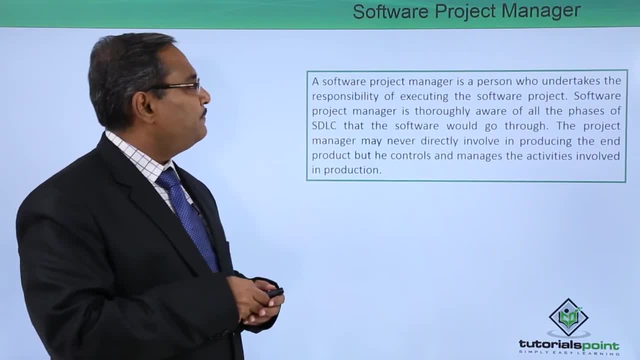 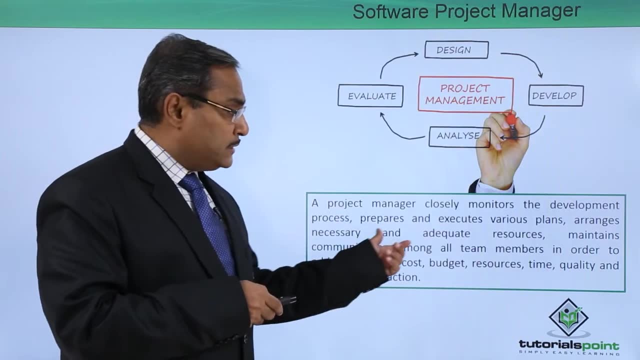 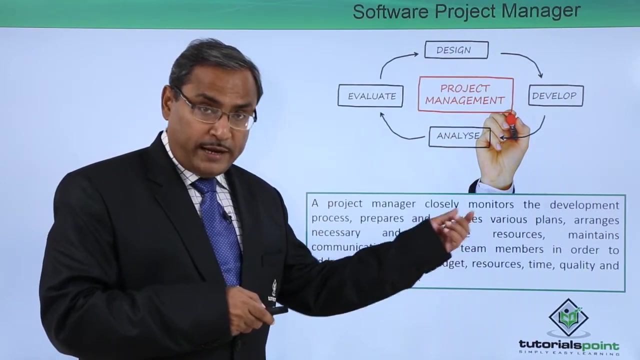 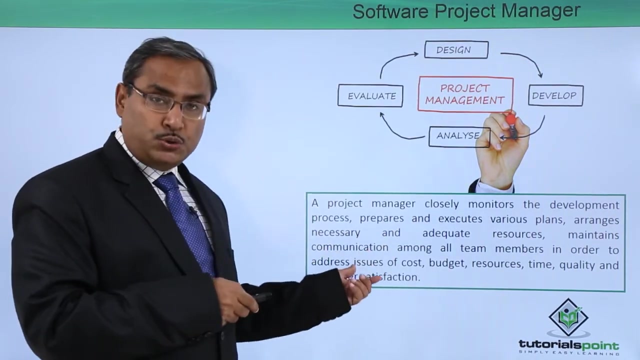 having supervision on all these aspects. A software project manager closely monitors the development process, prepares and executes various plans and arranges necessary and adequate resources And also very important, that maintains communication among all the team members in order to address some issues related with cost budget. 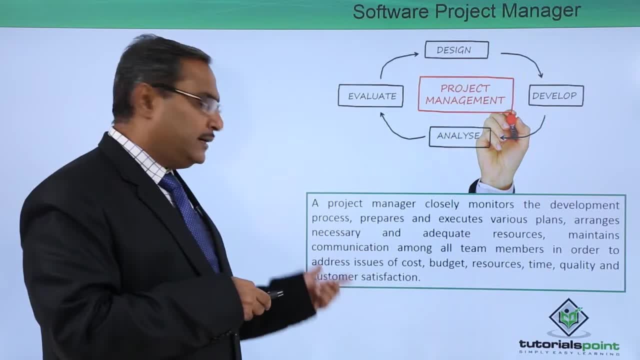 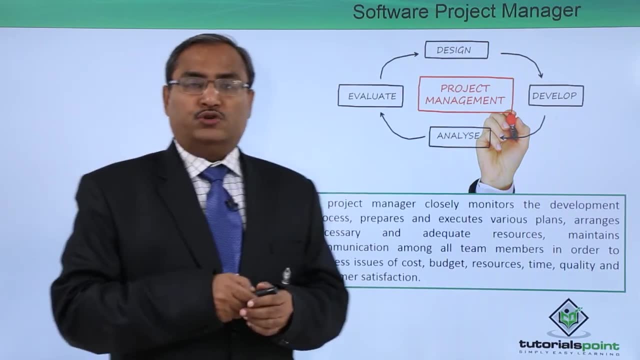 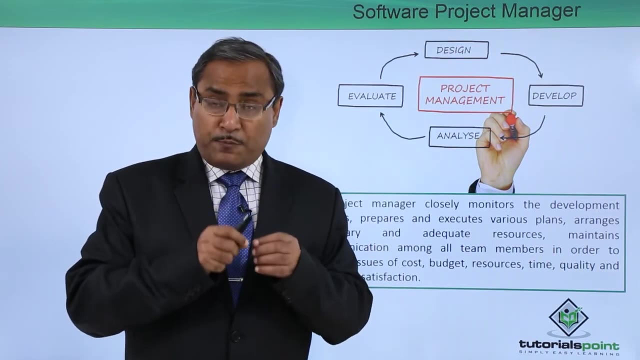 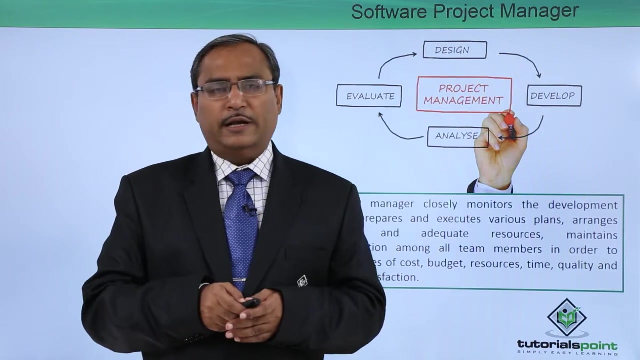 resources, time and quality and customer satisfaction. So these are the main purposes of one software project manager. So software project manager is having is performing multiple different responsibilities and a very important and vital role in the software development process. Now let us see what are the different responsibilities that one software 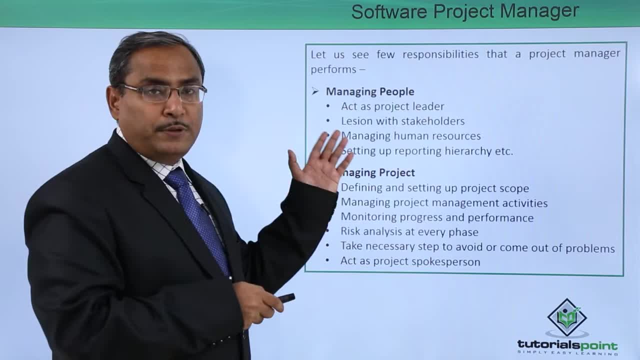 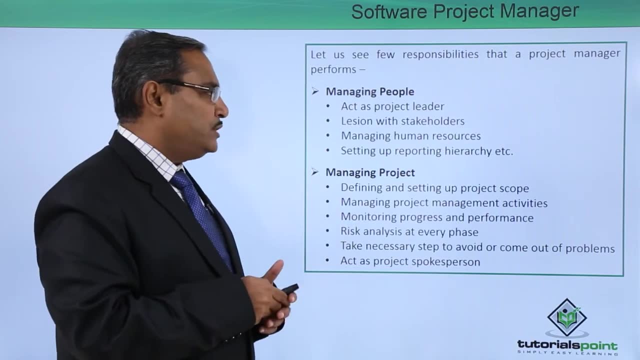 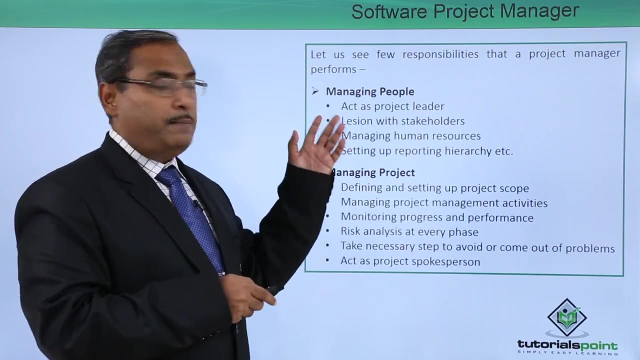 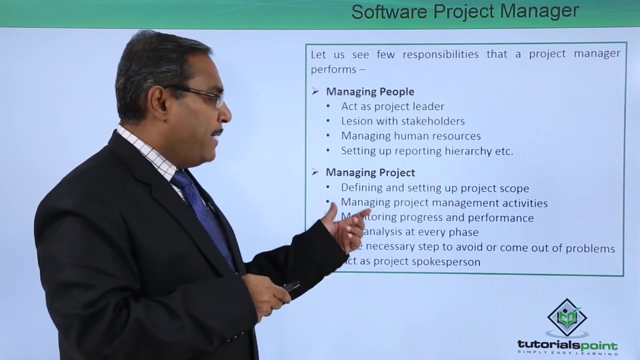 project manager will perform. So managing people, So act as a project leader, liaise with the stakeholders, managing human resources and setting up reporting hierarchy. So these are the different roles in case of managing people. Managing project we are having: defining and setting up project scopes and managing